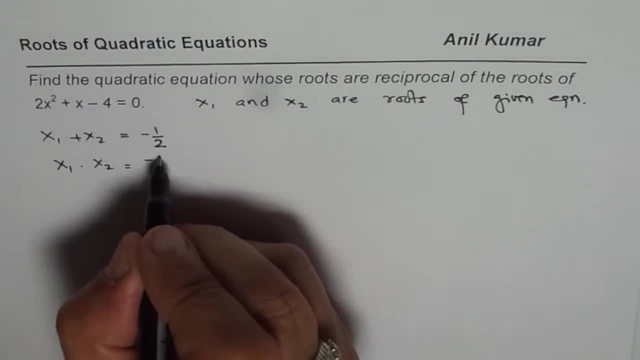 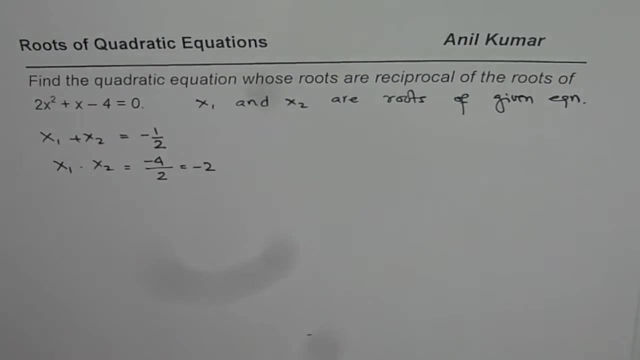 c over a, that is, in this case, c is minus 4 over a, which is 2, which will give us minus 2,. okay, How did we get this formula right? Basically, if you recall, quadratic equation. 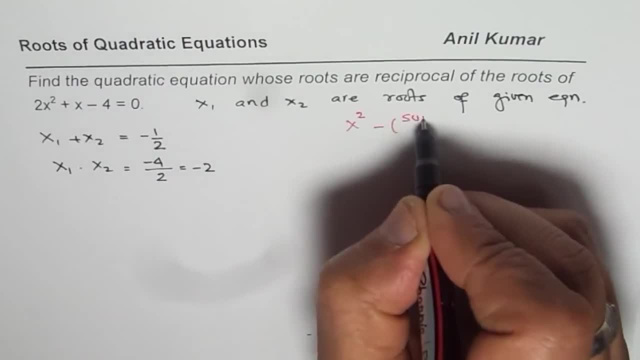 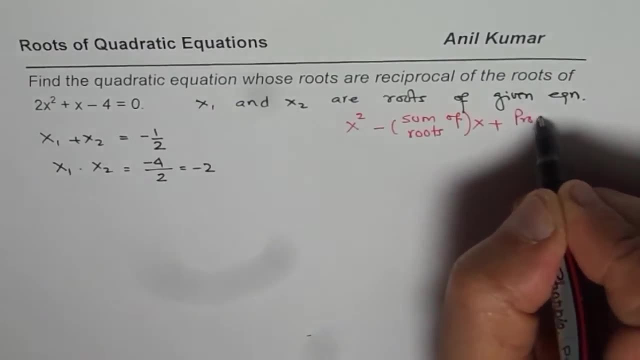 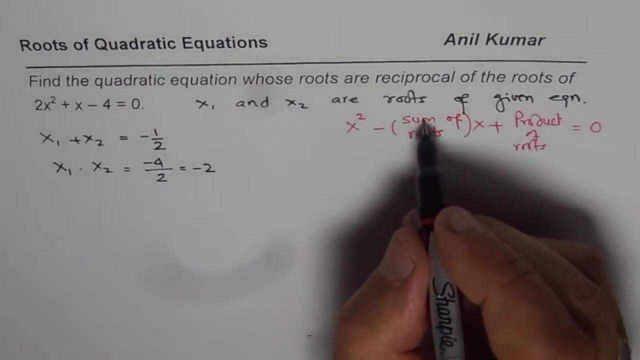 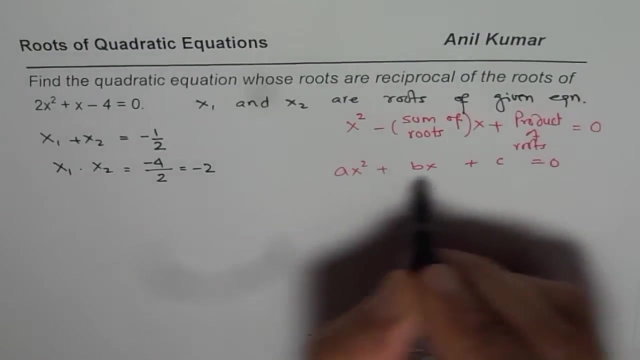 could be written as: x squared minus sum of roots, times x plus product of roots. A equals to 0, where sum of roots will be. let us write general equation: ax squared plus bx plus c equals to 0.. If I divide by a, I get: x squared plus b over ax plus c over a equals to 0.. So 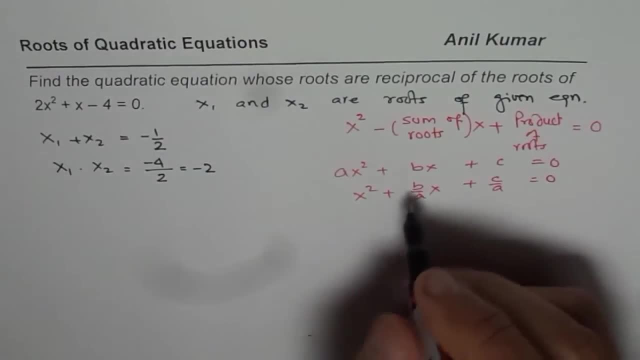 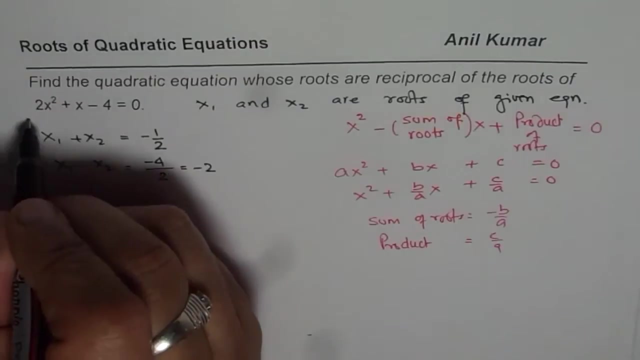 sum of roots, you can see, is minus b over a right. So we have sum of roots equals to minus b over a and product equals to c over a. So that is how we get In this equation: a equals to 2, b equals. 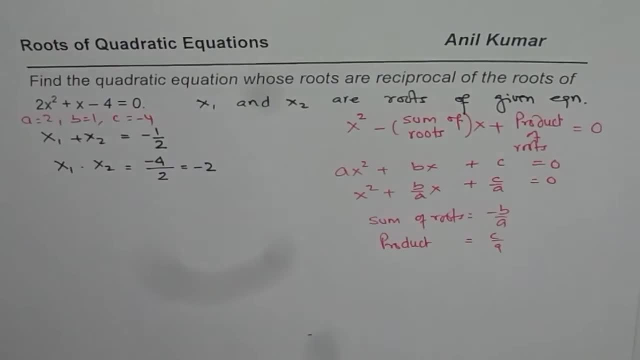 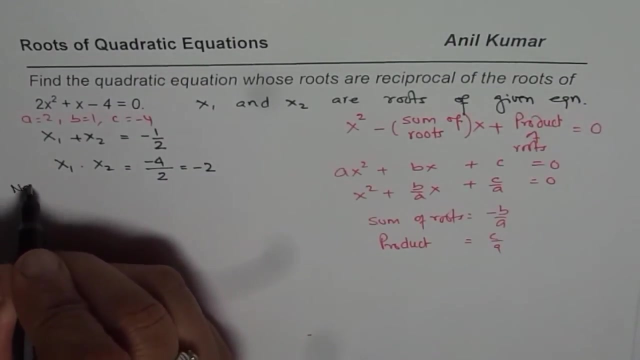 to 1 and c equals to minus 4.. So that is the background for the same. Anyway, now let us look into the question once again. It says: find the quadratic equation whose roots are reciprocal of the roots of this equation. So the new equation which we want to find, the roots are reciprocal. 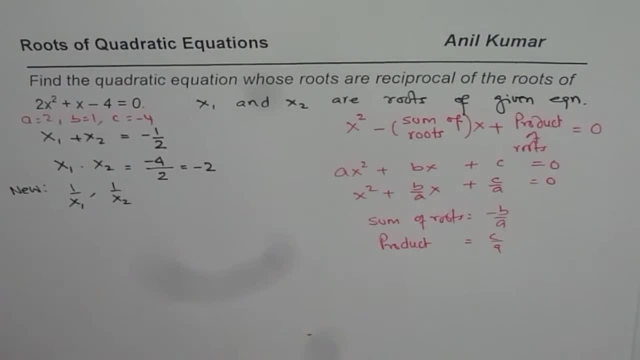 roots are 1 over x1 and 1 over x2, correct. Now, if these are the roots, then what is their product? Then the product is 1 over x1 times 1 over x2, which is 1 over x1, x2, right Now, we know x1. 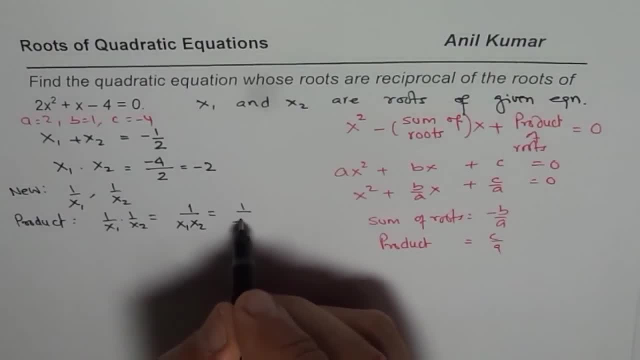 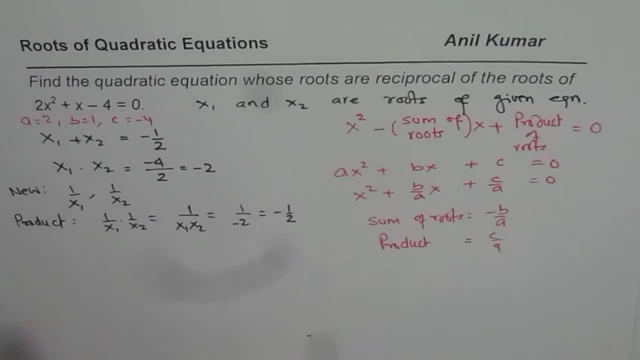 times x2 is minus 2.. So this should be 1 over minus 2, or it is minus half. So product of roots is minus half. So we get this part of the equation correct. Let us find the sum now. Sum of the roots. 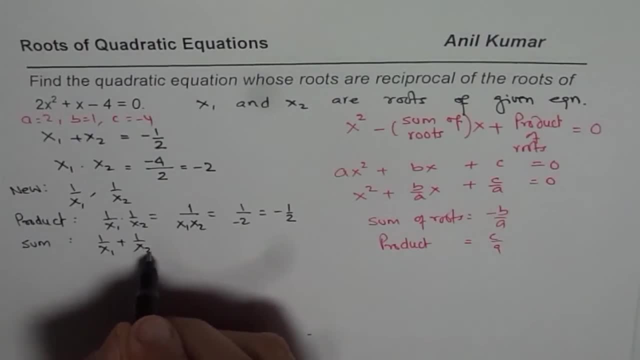 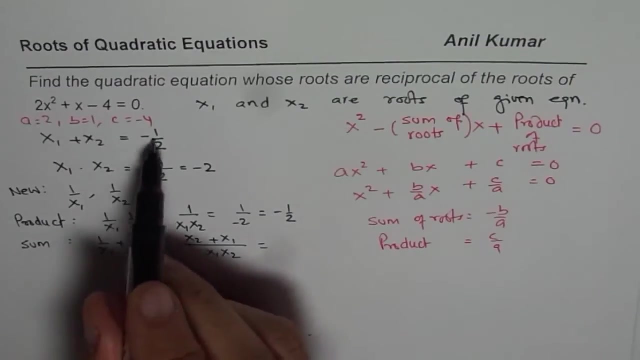 will be 1 over x1 plus 1 over x2.. So what we can do is we can take common denominator, So we get x1, x2 and x2 plus x1 in the numerator. Now x2 plus x1 is same as x1 plus x2, which is minus half.